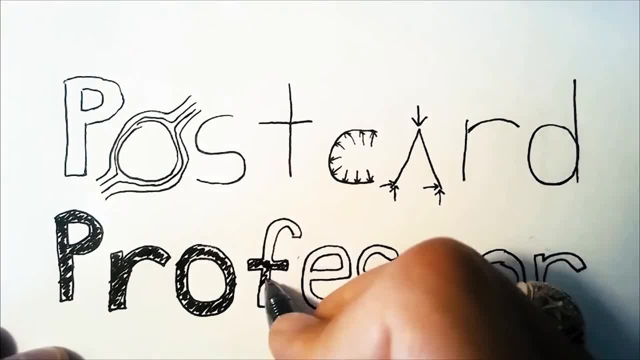 Hello and welcome to The Postcard Professor, where we take complex ideas and explain them in the space of a postcard. 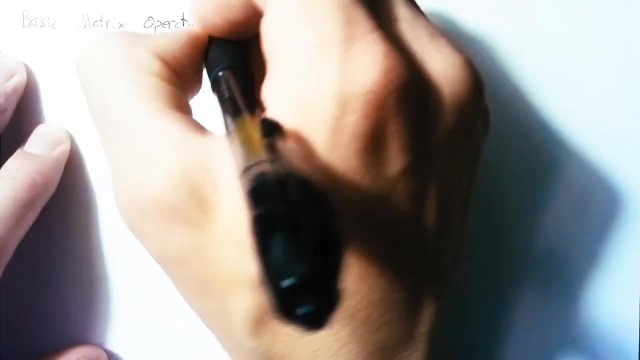 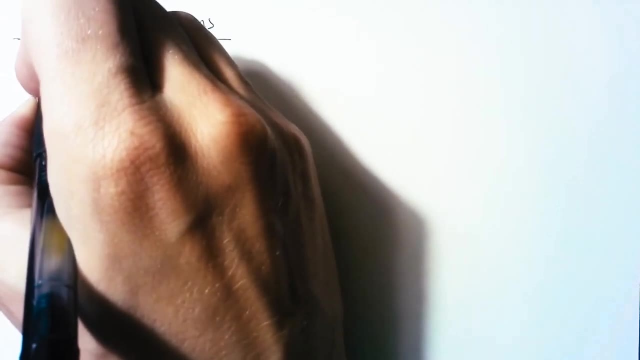 This video will be a review of basic matrix operations. We're going to cover four different operations here and then on top of that I just want to have a small note on how we define these. 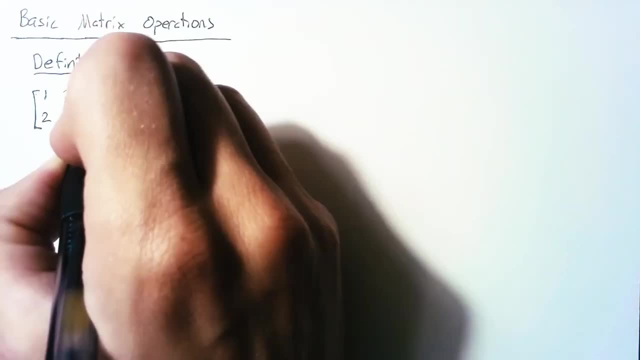 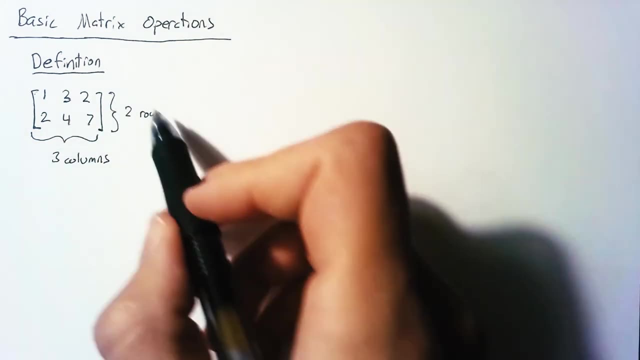 So for matrix definition, let's say we have some matrix. This matrix has a number of rows and a number of columns and with these two pieces of information we define the shape 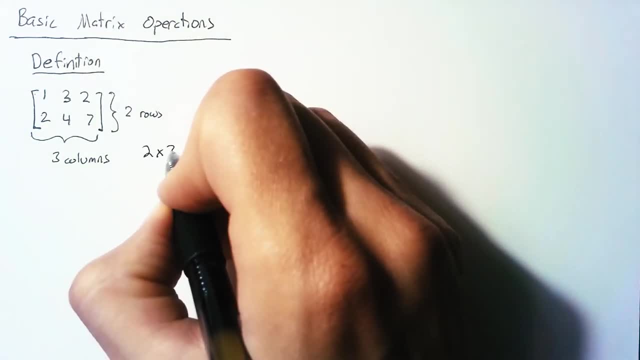 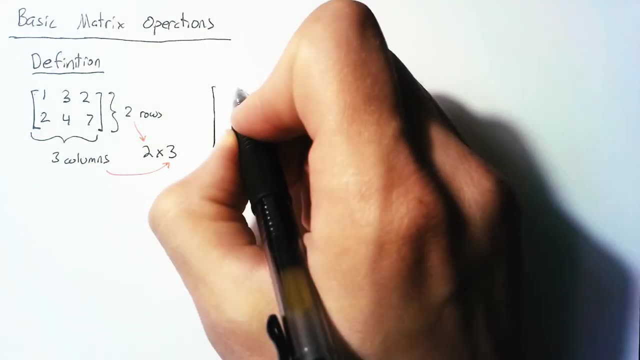 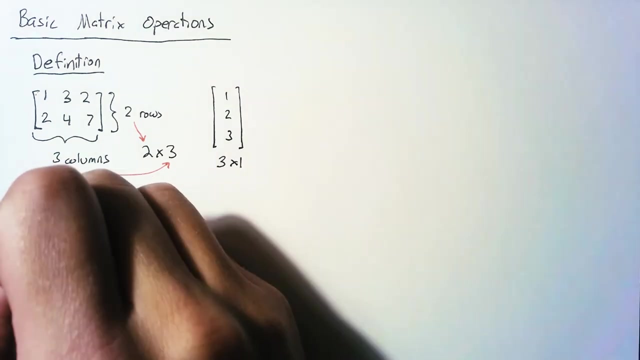 of the matrix. This is a two by three matrix just from the two rows and three columns. If we have a matrix that is three rows and one column this is just a three by one matrix. Now the first 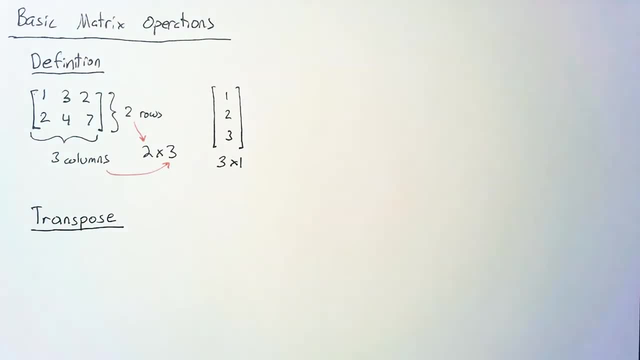 operation we're going to talk about is called the matrix transpose and all the matrix transpose are called matrix transpose. All the matrix transpose are called matrix transpose because they're called matrix transpose. The matrix transpose does is change the shape of the matrix by flipping it. 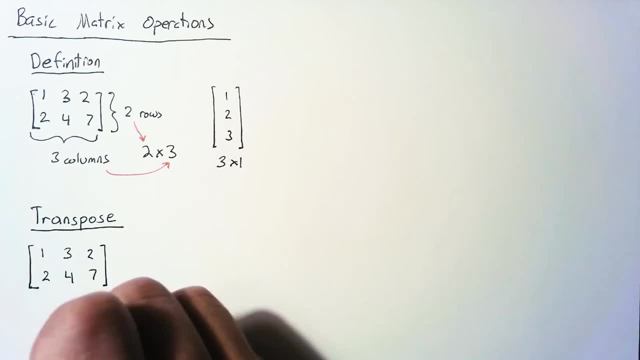 So if we have our same matrix as before which is a two by three we can transpose that matrix in order to end up with a three by two matrix. So the way this works the first element stays the same but then for the second element in the row we actually look to the second element in the column 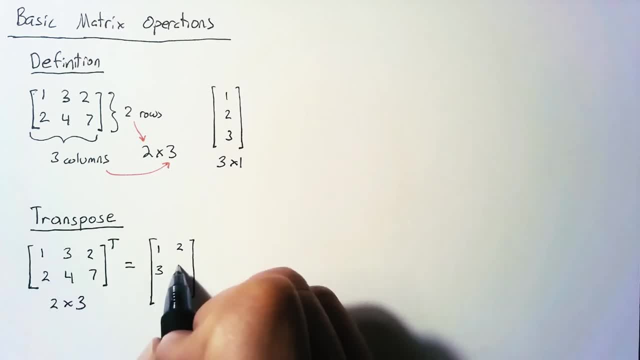 and so we get the one and the two then we get the three and the four and then finally the two and the seven and this is now a three by two matrix so three rows and two columns. So next 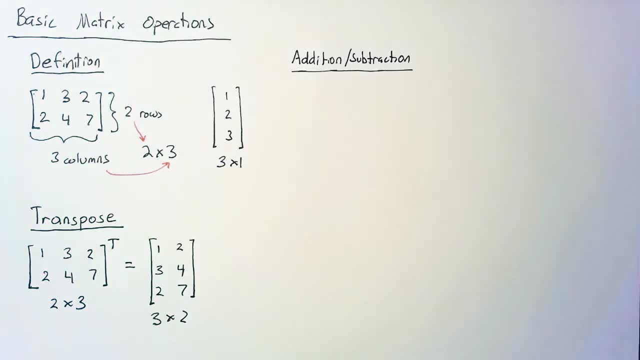 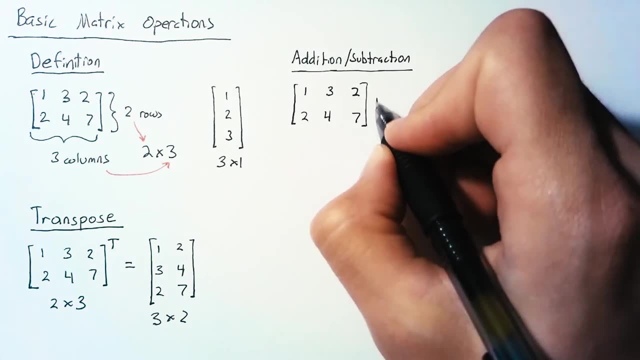 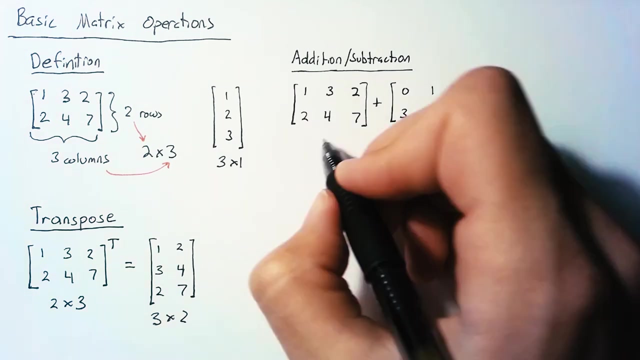 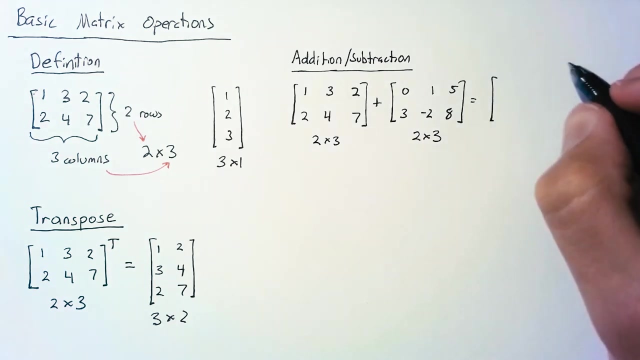 let's look at addition and subtraction. These are essentially the same thing of course but the basic idea is that for addition and subtraction we just look element by element. So we have to add and subtract matrices that have the exact same shape meaning that if this matrix here is a 2x3 the matrix that we're going to add is a 2x3. The matrix that we're adding to it also has to be a 2x3 and we're going to end up with a 2x3. 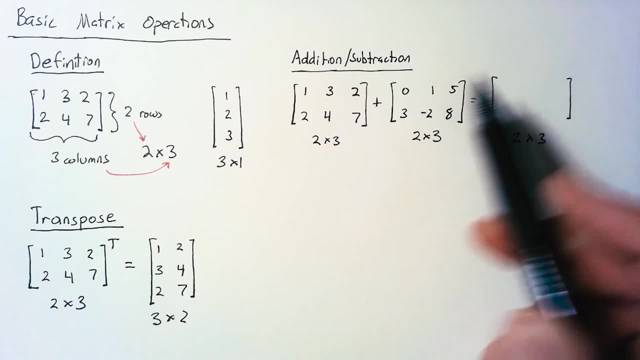 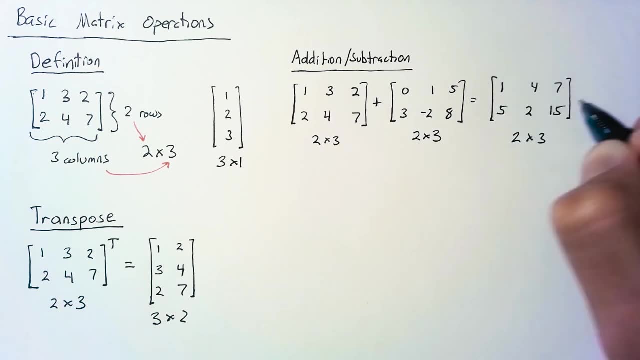 And to get the values here we just add the first element to the first element so one plus zero is one three plus one is four two plus five is seven and so on. Now the next one is multiplication 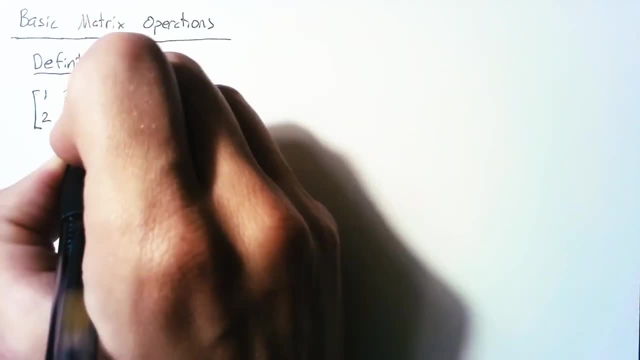 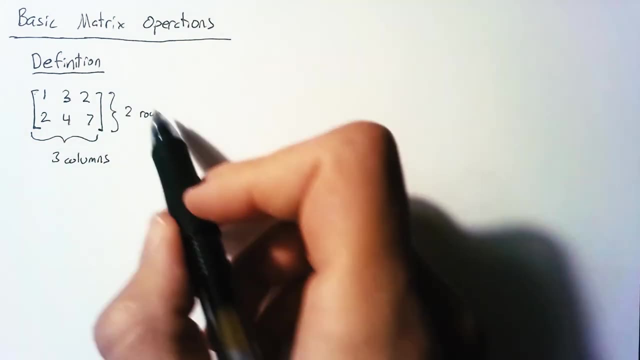 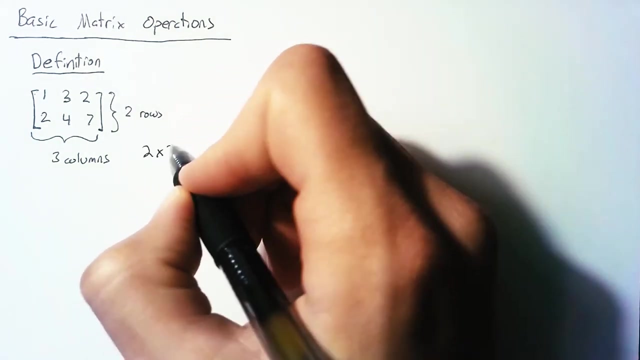 So for matrix definition, let's say we have some matrix. This matrix has a number of rows and a number of columns And with these two pieces of information we define the shape of the matrix. This is a 2x3 matrix, just from the two rows and three columns. If we have a matrix, 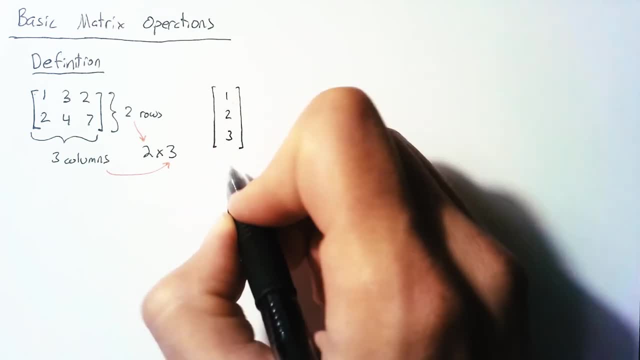 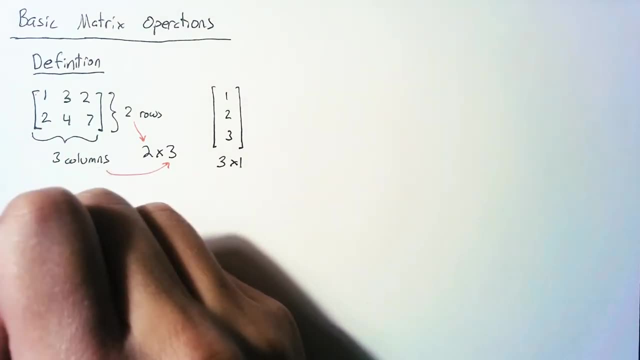 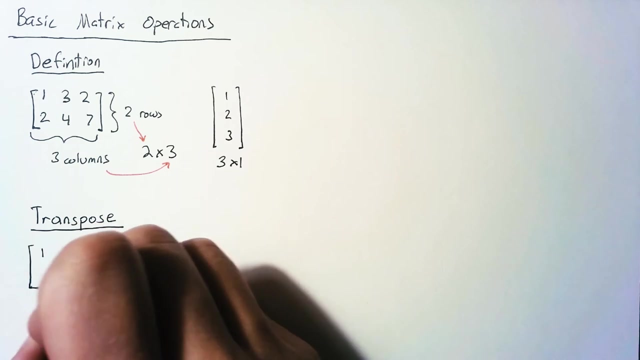 that is three rows and one column. this is just a 3x1 matrix. Now the first operation we're going to talk about is called the matrix transpose, And all the matrix transpose does is change the shape of the matrix by flipping it. So if we have our same matrix as before, 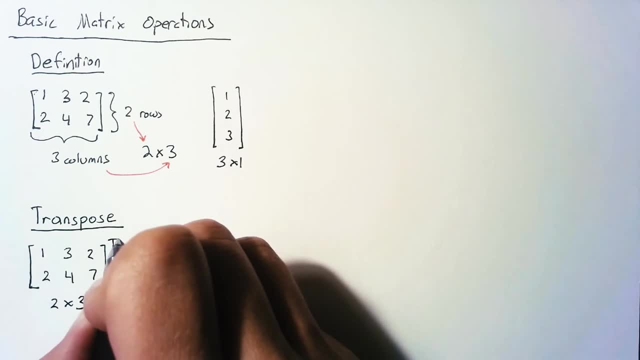 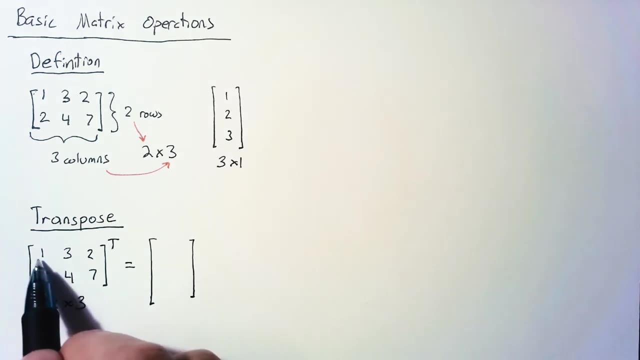 which is a 2x3,, we can transpose that matrix in order to end up with a 3x2 matrix. So the way this works, the first element stays the same, but then, for the second element in the row, we actually look to the second element in the column, And so we get the 1 and the 2,. 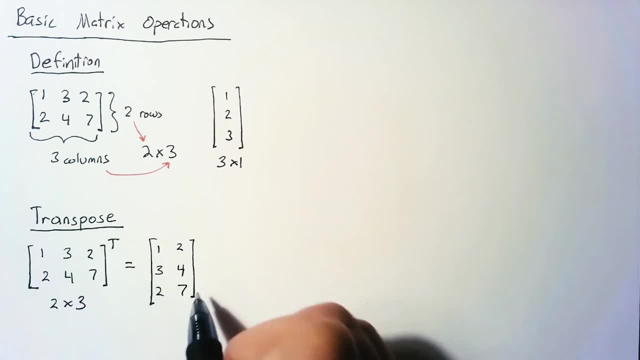 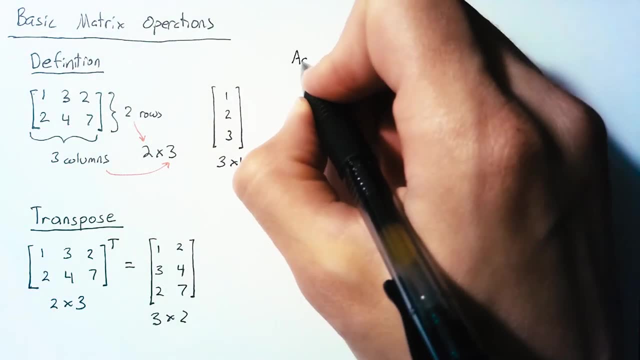 then we get the 3 and the 4, and then finally the 2 and the 7. And this is now a 3x2 matrix, So three rows and two columns. So next let's look at addition and subtraction. These are essentially the same thing, of course. 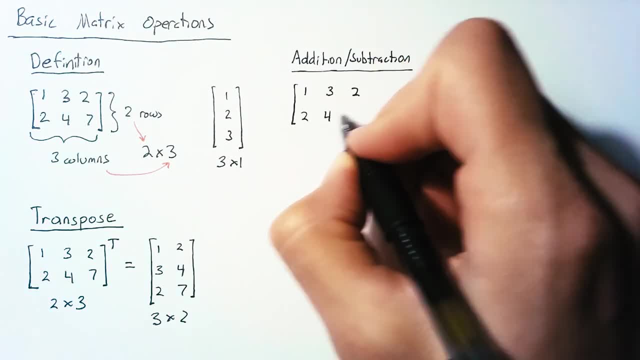 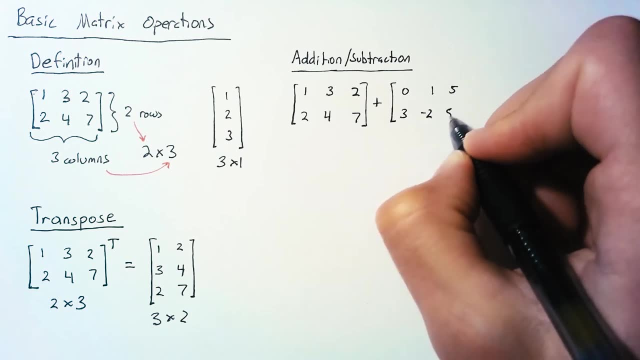 but the basic idea is that for addition and subtraction we just look element by element, So we have to add and subtract matrices that have the exact same shape, Meaning that if this matrix here is a 2x3, the matrix that we're 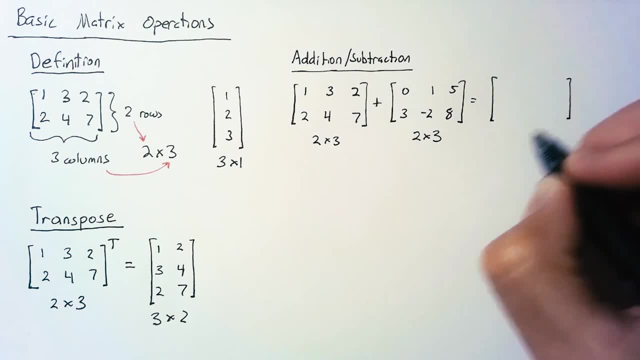 adding to it also has to be a 2x3. And we're going to end up with a 2x3. And to get the values here, we just add the first element to the first element. So 1 plus 0 is 1,. 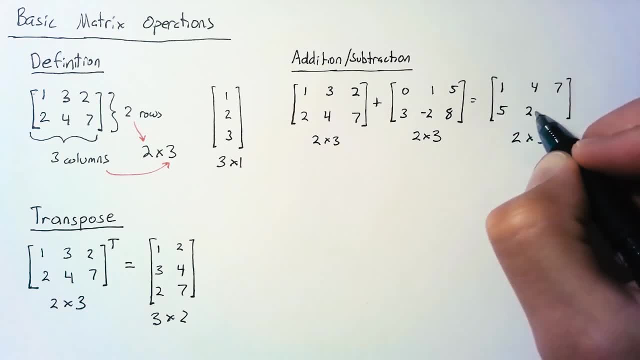 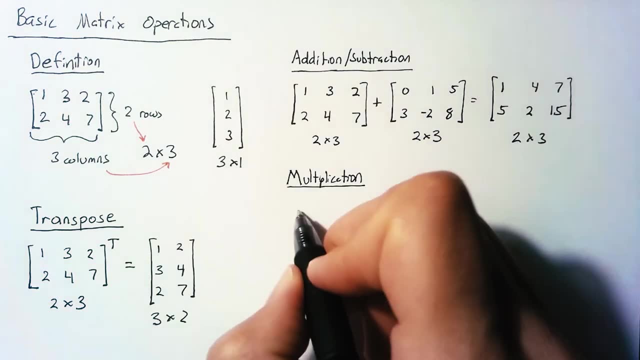 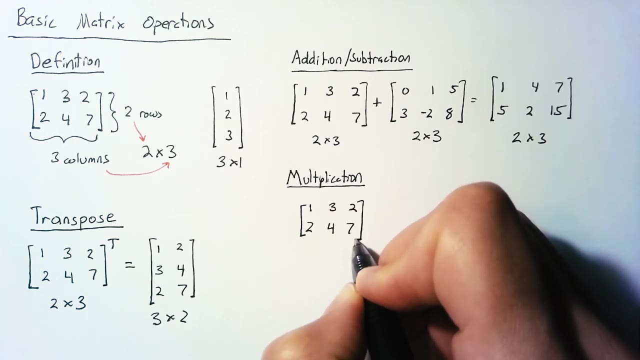 3 plus 1 is 4,, 2 plus 5 is 7, and so on. Now the next one is multiplication, and this might be the most important, But with multiplication we have some stronger rules as to what matrices we can actually multiply together. So let's take that. 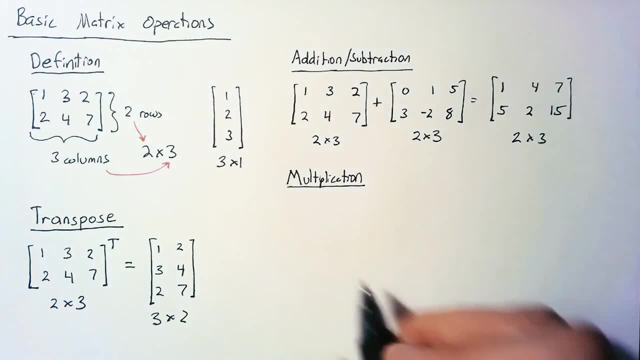 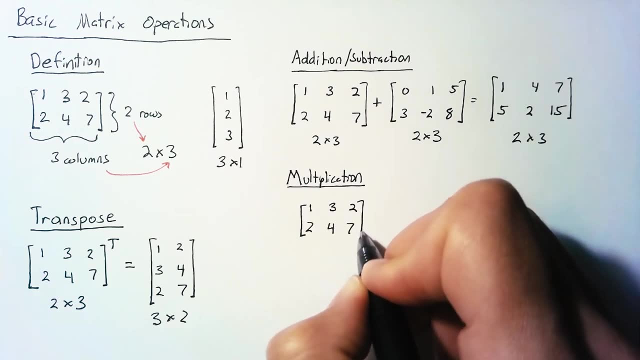 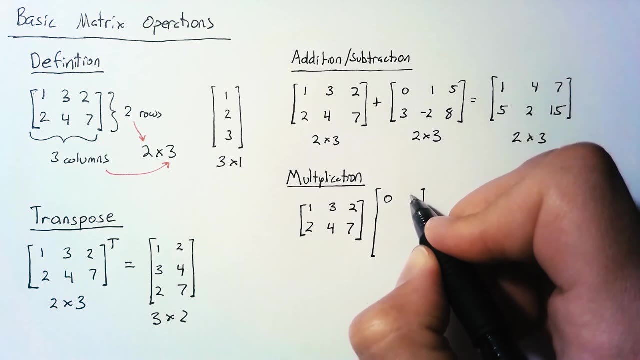 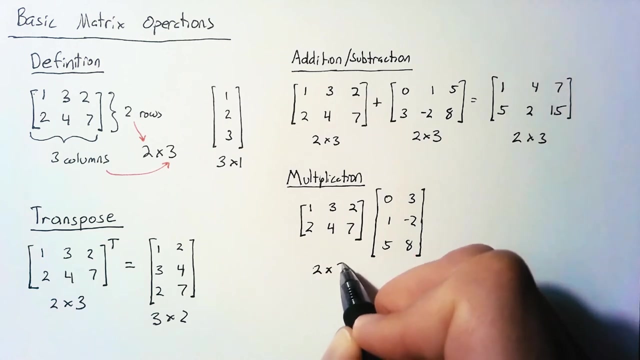 and this might be the most important but with multiplication we have some stronger rules as to what matrices we can actually multiply together. So let's take that same matrix as before and we're going to multiply it by the transpose of the same second matrix as before. So the rule here is that if we have a 2x3 matrix we have to match that 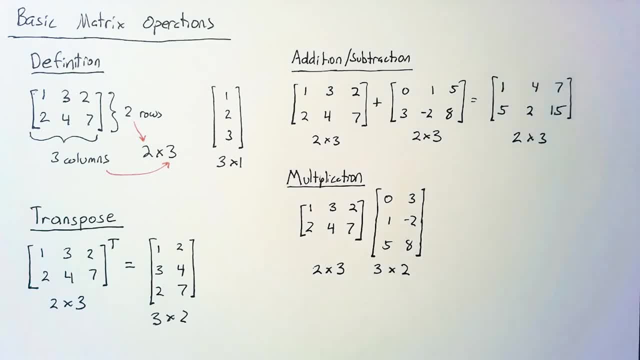 with a three by something matrix. So the important part of that is the number of columns of the first matrix has to match the number of rows of the second matrix. The three by three here these must match. And what we end up with is a two by two matrix and really what you end up with is whatever's left over from these two is going to be the shape of the new matrix. Now as for what's in these elements 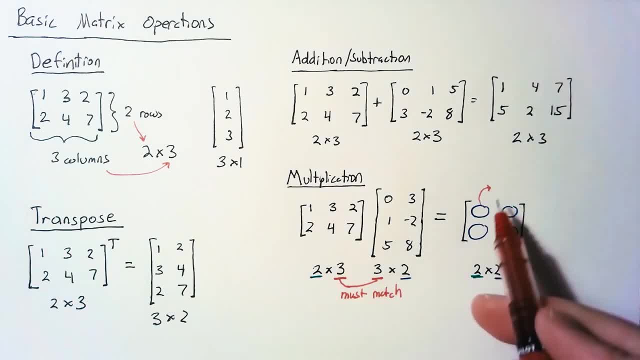 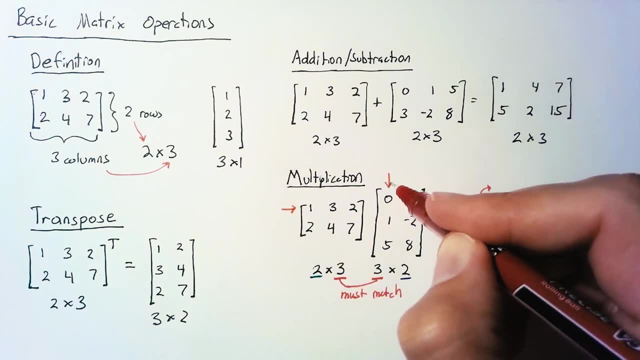 let's start with the first element. The way we work this is we take the elements of our first row and our first column and we multiply each of those elements together. 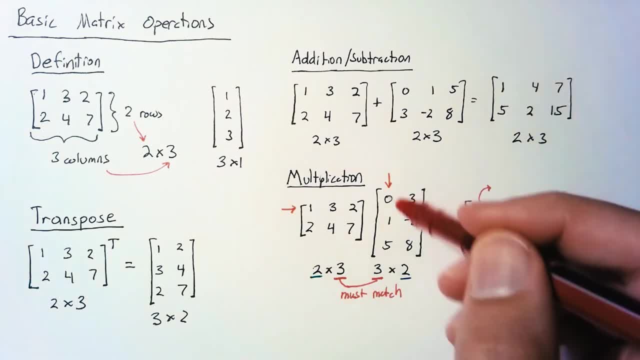 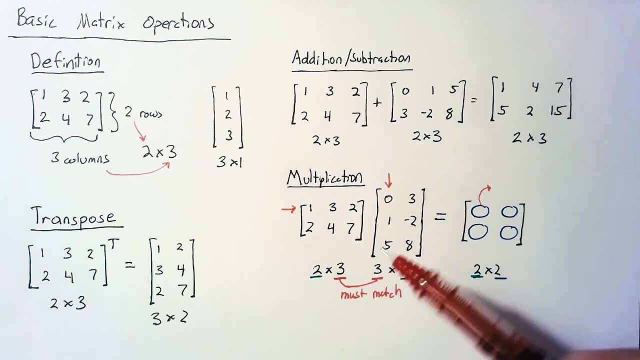 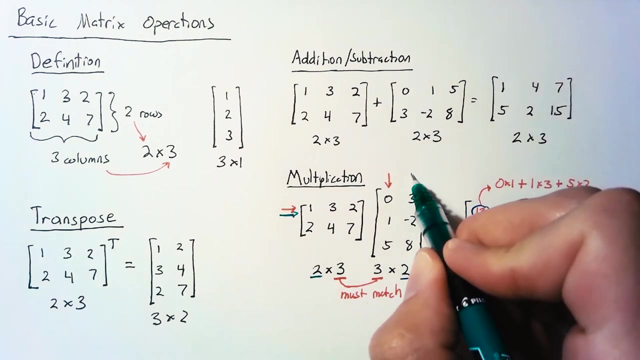 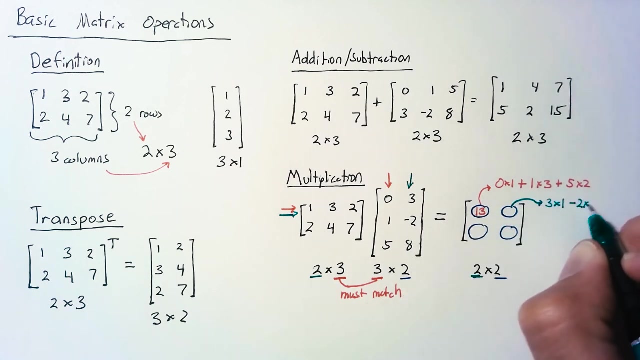 So we take the three by three and we multiply the value of those elements and then we plug them together. And we're going to match and actually sum up the numbers. And that's why these values must match. We're gonna take these three and then just push them over and lay them on top of these top three. So we're gonna end up with zero times one because that's this first element plus one times three and then finally plus five times two. the row we're still in the first row so we're going to keep to the first row for the first matrix but then we're in the second column now and so we're going to look at the second column of our second matrix so now what we end up with is 3 times 1 minus 2 times 3 plus 2 times 8 plus 8 times 2. so we have 16 minus 6 is 10 plus 3 is 13 and so we end up with 13 again for the bottom left 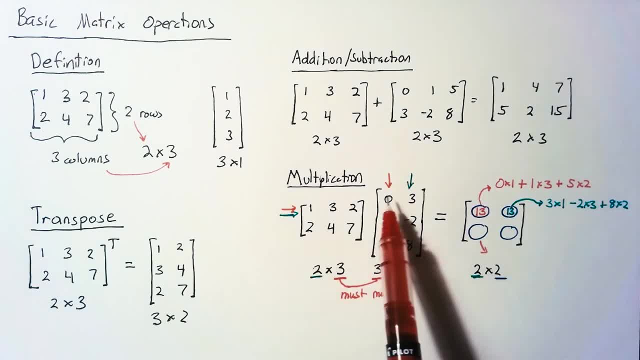 now we're looking at the second row and the first column so we end up with 0 times 2 which is 0 1 times 4 is 4 and then 7 times 5 is 35 so we end up with 39 for that so we end up with 39 for that element then finally we're looking at the second 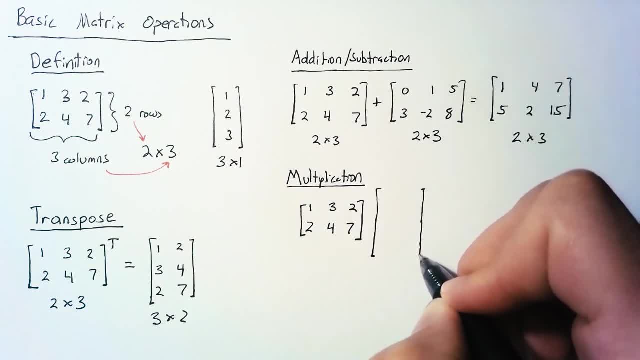 same matrix as before and we're going to multiply it by the transpose of the same second matrix as before. So the rule here is that if we have a 2x3 matrix we have to match that with a 3x something matrix. So the important part of that is the number of columns of the first matrix has to. 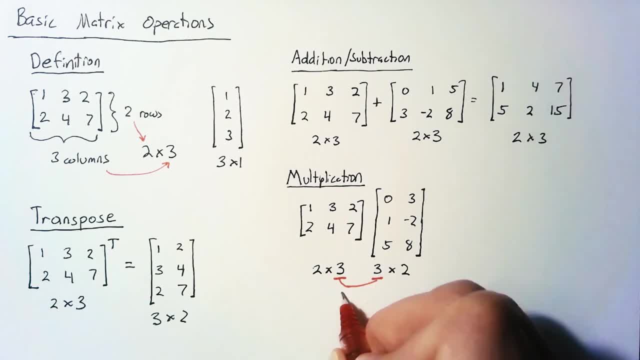 match the number of rows of the second matrix, The 3x3 here. these must match And what we end up with is a 2x2 matrix, And really, what you end up with is whatever's left over from these two is going to be the shape of the new matrix. Now, as for what's in these elements, 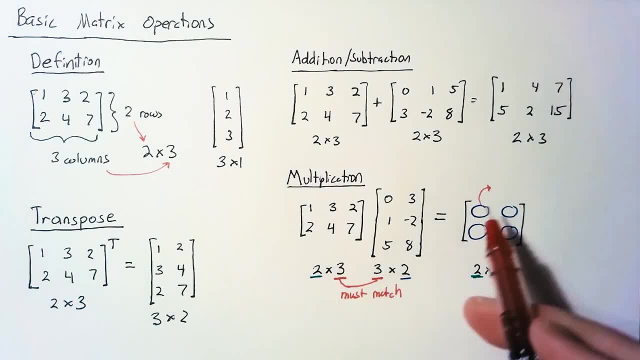 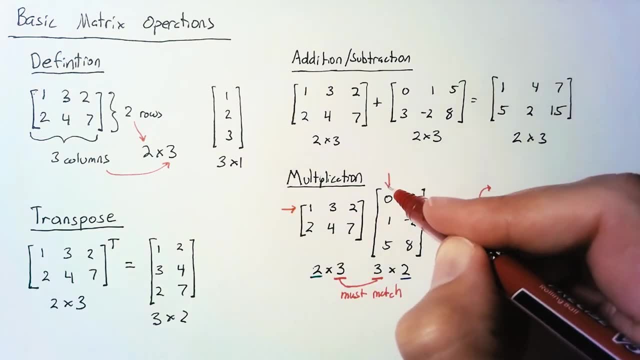 let's start with the first element. The way we work this is: we take the elements of our first row and our first column and we multiply each of those elements together. That's what we're going to do here: We're going to multiply each of those elements together. 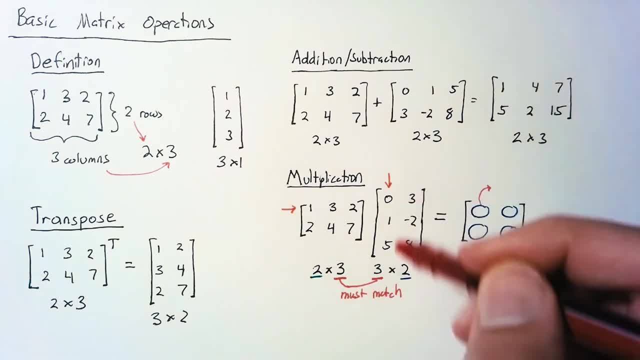 That's what we're going to do here. We're going to multiply each of those elements together, And that's why these values must match. We're going to take these three and then just push them over and lay them on top of these top three, So we're going to end up with 0 times 1,. 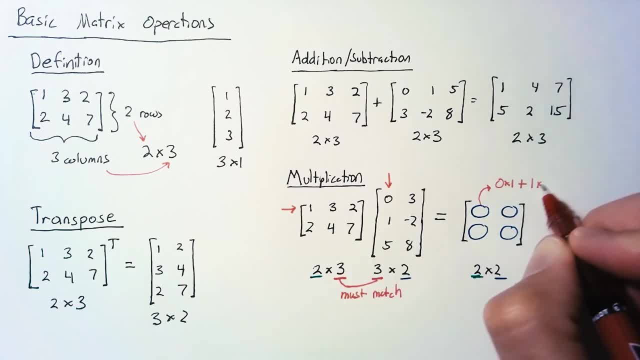 because that's this first element plus 1 times 3, and then finally plus 5 times 2.. So the end result there we get: 3 plus 10 is 13.. For the next one we look at the row: We're still in the first. 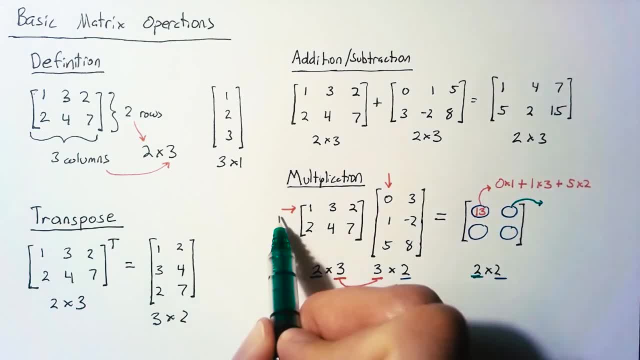 row. So we're going to keep to the first row for the first matrix, but then we're in the second column now, And so we're going to look at the second column of our second matrix. So now what we end up with is 3 times 1 minus 2 times 3 plus 2 times 8 plus 8 times 2.. So we have 16 minus 6 is 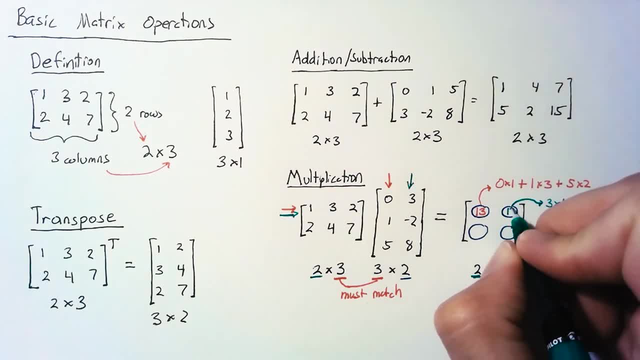 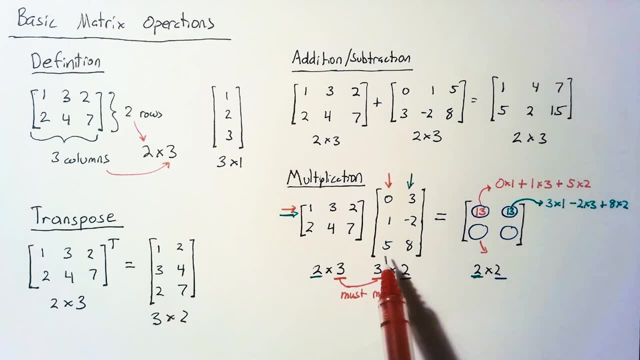 10 plus 3 is 13.. And so we end up with 13 again For the bottom left. now we're looking at the second row and the first column, So we end up with 0 times 2, which is 0.. 1 times 4 is 4.. And then 7. 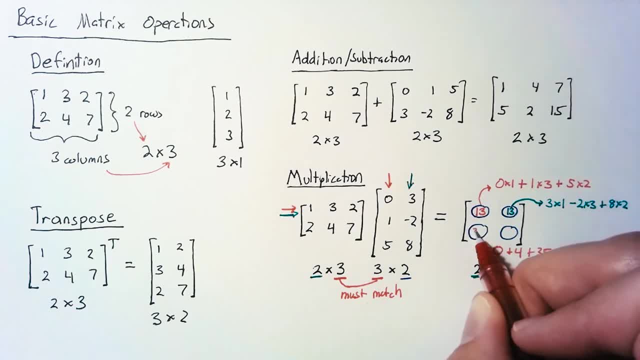 times 5 is 35.. So we end up with 39 for that. So we end up with 39 for that element. Then, finally, we're looking at the second row and the second column. So we have 3 times 2 is 6.. 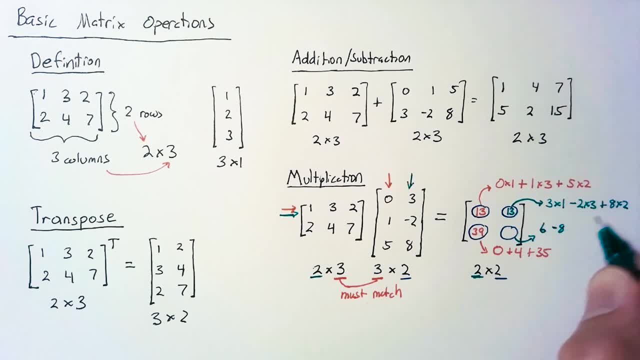 Negative. 2 times 4 is negative 8.. And then 8 is 8. Times 7 is 56. So we end up there with 54.. The final operation I want to talk about is the inverse of a matrix. Now there are operations that we can reasonably perform for 2 by 2 and 3. 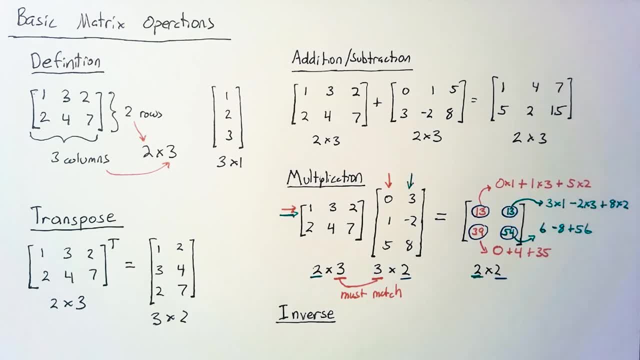 by 3 matrices, But honestly, it's probably easier just to use substitution for those matrices. if you're going to be doing it by hand, Really what you'll be doing is using some computational tool, such as Python or MATLAB, in order to invert the matrix. If we have a matrix, 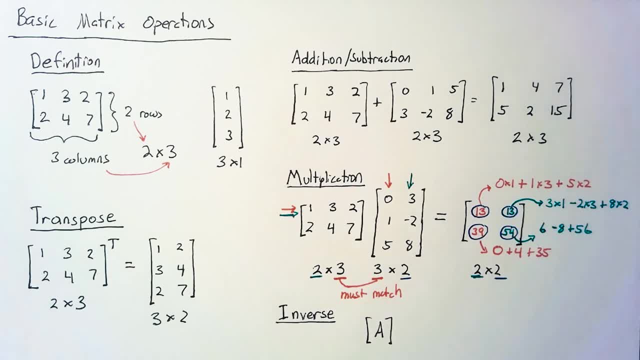 right, let's say we have a matrix And I'm going to call this matrix A. This stands for a square matrix, which means that the number of rows equals the number of columns. The matrix inverse multiplied by the matrix becomes the identity matrix. And if you take the identity, 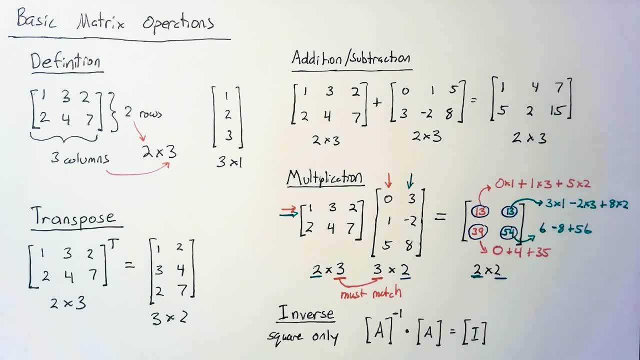 matrix and multiply it by a vector or another matrix, then it just disappears. This identity matrix is going to be equal to just 1s on the diagonal and 0s everywhere else, And that will continue on forever. But let's say that this is a 4 by 4. And so we end up with 1s on the diagonal. 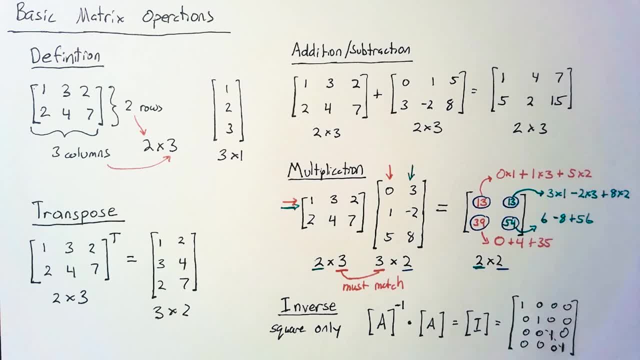 and then 0s everywhere else. And the reason we use this so much is that we end up with systems equations- which we'll cover in the next video- And we need to get rid of some matrix that's pre-multiplying a vector, And so we'll multiply by the inverse to get rid of it. So that's a quick overview of 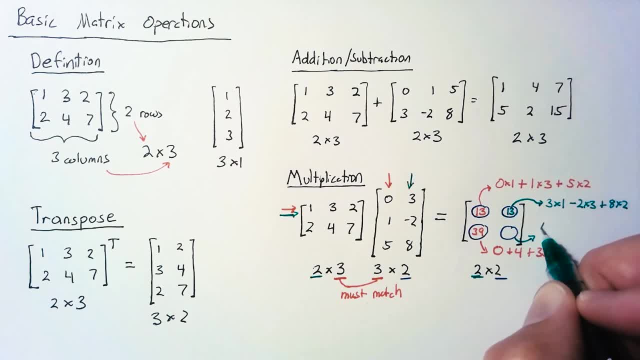 row in the second column so we have 3 times 2 is 6 negative 2 times 4 is negative 8 and then 8 times 7 is 56. so we end up there with 54. the final operation i want to talk about is the inverse of a matrix now there are operations that we can reasonably perform for 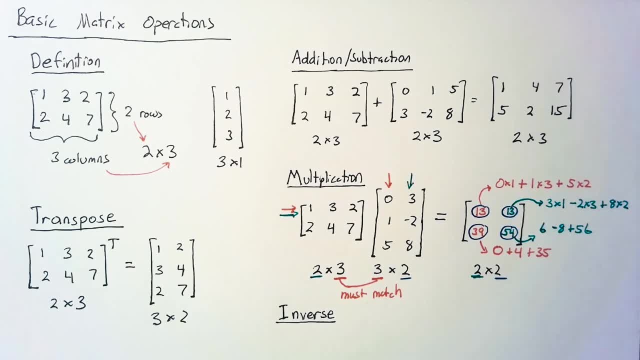 2 by 2 and 3 by 3 matrices but honestly it's probably easier just to use substitution for those matrices if you're going to be doing it by hand really what you'll be doing is using some 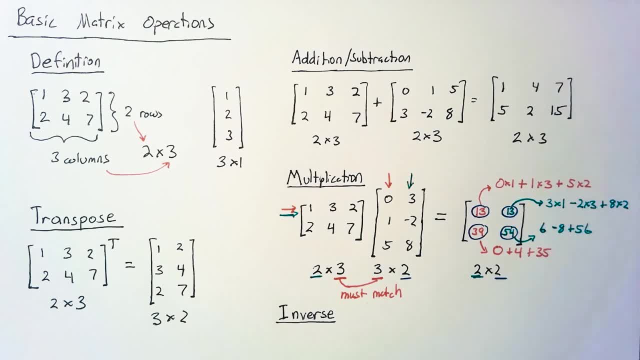 tool such as python or matlab in order to invert the matrix if we have a matrix right let's say we have a matrix and i'm going to call this matrix a this this stands for a square matrix which means that the number of rows equals the number of columns the matrix inverse multiplied by the matrix becomes the identity matrix and if you take the 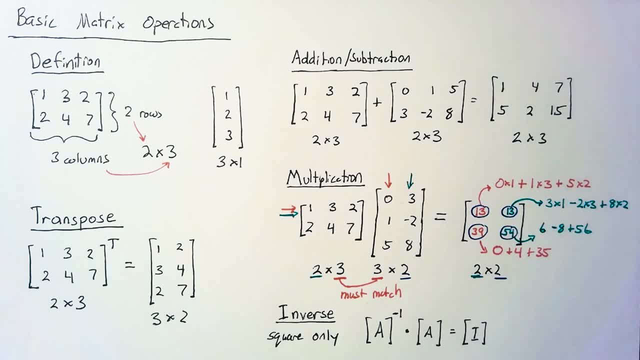 identity matrix and multiply it by a vector or another matrix then it just disappears this identity matrix is going to be equal to just ones on the diagonal and zeros everywhere else and that will continue on forever but let's say that this is a 4 by 4 and so we end up with ones 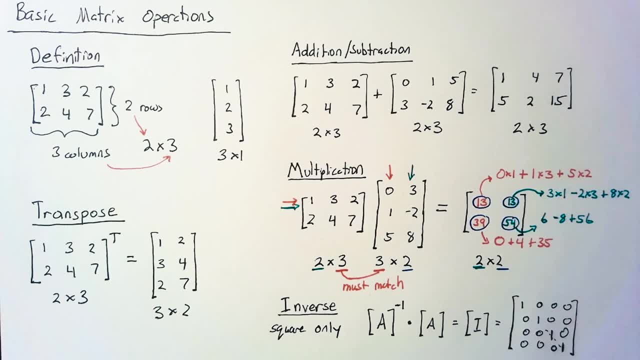 on diagonal and then zeros everywhere else and the reason we use this so much is that we end up with less than one fourth of a factor and that's because we already have a dimension matrix 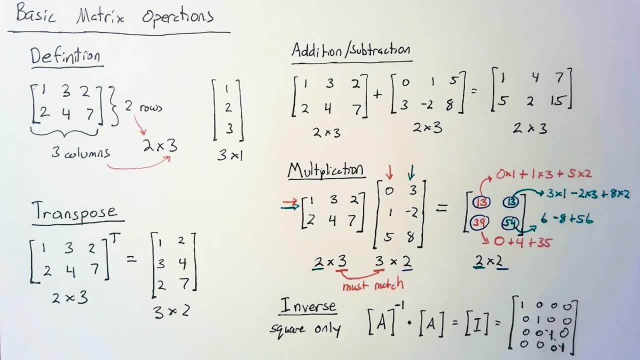 that's going to stop when we divide it by a vector so we want to make sure that we get rid of a vector and this is a great idea so let's go to machine learning and we're going to look at this equation so we'll have some equations which we'll cover in the next video and we need to get rid of some 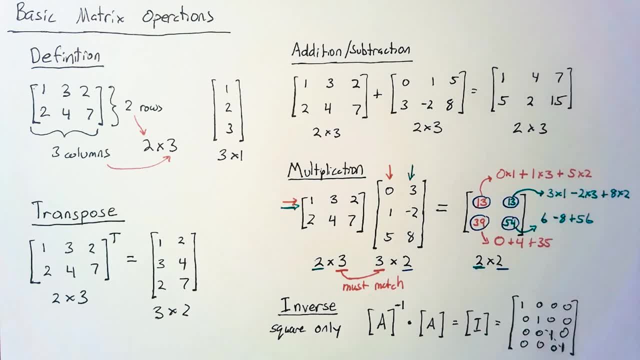 matrix that's pre-multiplying a vector and so we'll multiply by the inverse to get rid of it so 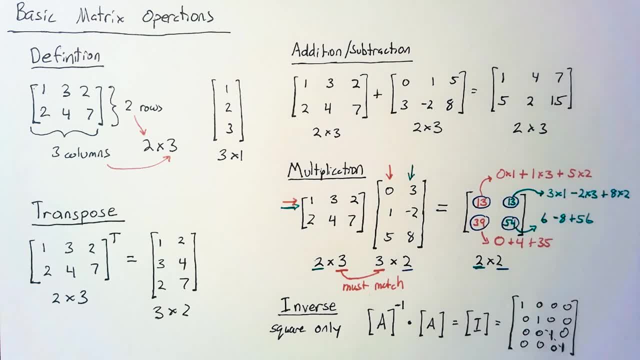 matrix operations. We'll go in more in depth a little bit as we get into the system of equations in matrix form, because what we're actually going to be doing there is using these inverses in order to solve a system of equations. So we're going to be using these inverses in order to solve a system. 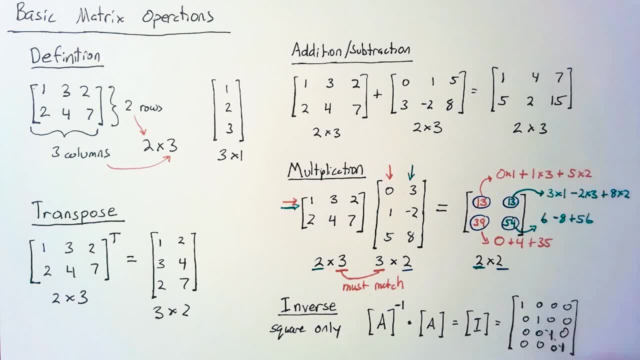 of equations, So we're going to be using multiplication and inverse directly there. In any case, I hope this was informative and I will catch you next time. 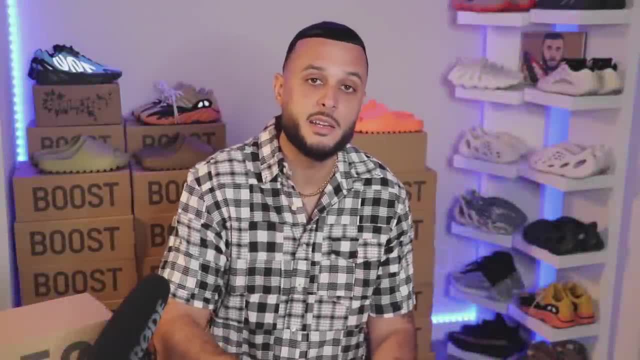 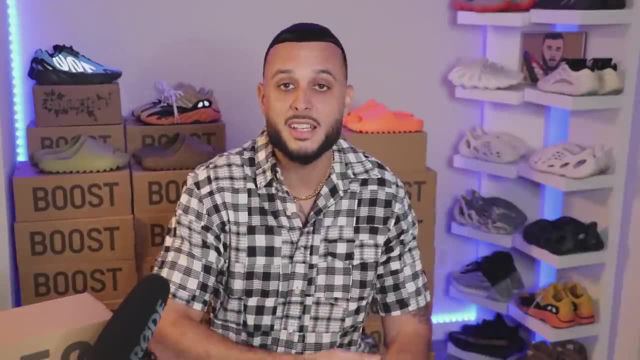 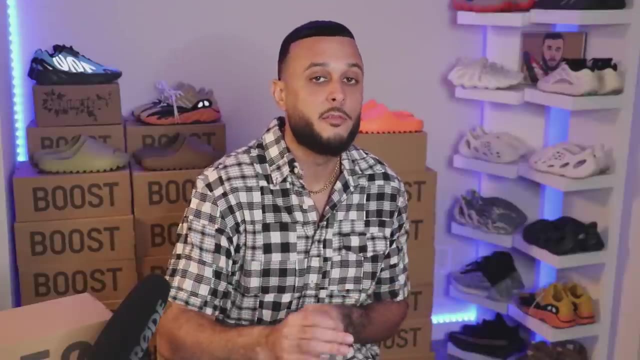 So it's safe to say that the Yeezy brand has had the biggest impact this summer in terms of sneaker releases. I mean, just look at the month of June alone: Some great drops from the bright cyan to the orange slides, all the way to the inflame amber 700.. Now we already know that. the month of March, 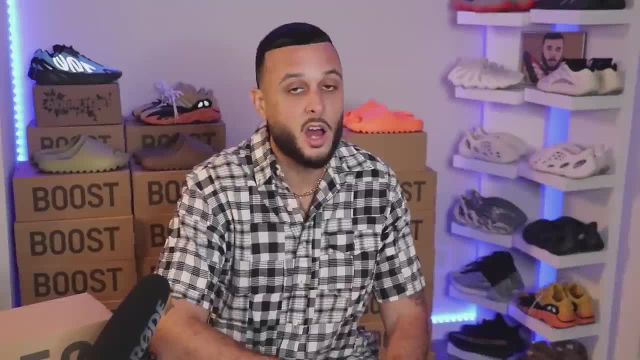 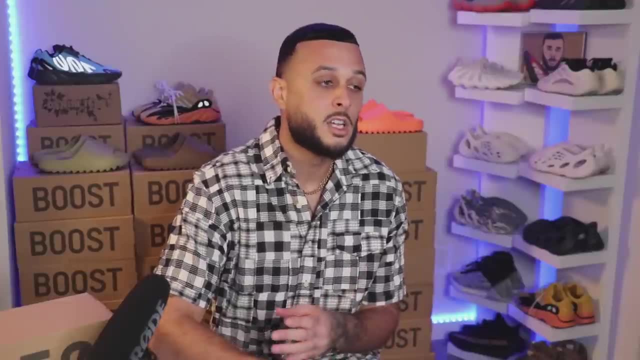 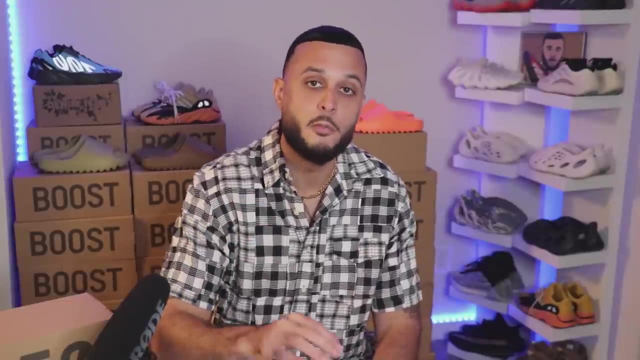 probably was the best month in terms of Yeezy releases. We saw the cloud white 450 debut, They dropped the 700 v2 creams as well as the foam runners, just to name a few. So I want to ask all of you guys: is June's releases touching, coming even close to what we saw from March? I think. 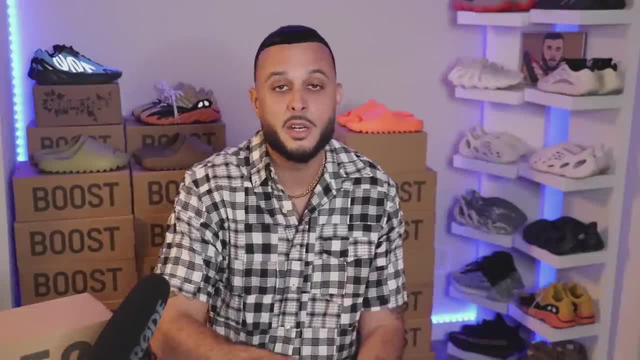 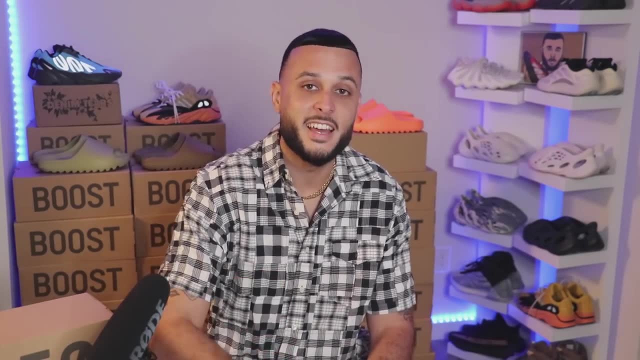 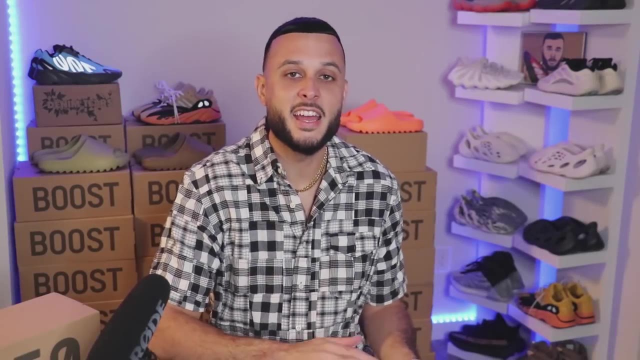 today's video will be very helpful in determining that situation. So, without further ado, let's get straight into the review of the Yeezy 450 dark slate. So what's good guys? JA, appreciate everybody for tuning in for today's new video. I'm going to continue the campaign. If you guys watch the. 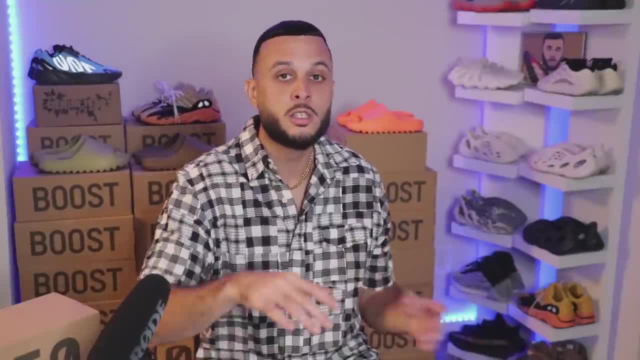 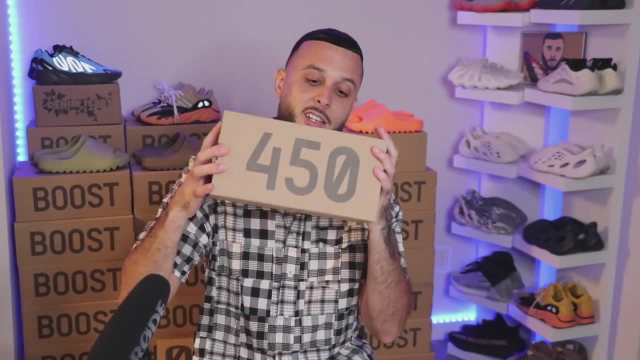 videos and you have not subscribed yet. it's kind of rude. Subscribe to the channel. This is now going to be the third early look in a row, So we're going to be taking a look at the Yeezy 450 dark slate, which is actually the second colorway of the Yeezy 450, which debuted back in March with. 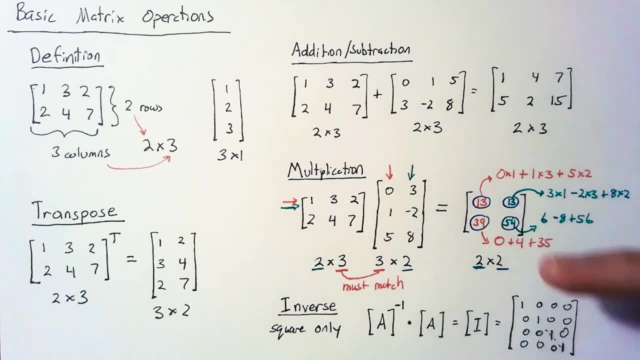 in order to solve a system of equations. So we're gonna be using multiplication and inverse directly there. In any case, I hope this was informative and I will catch you next time.